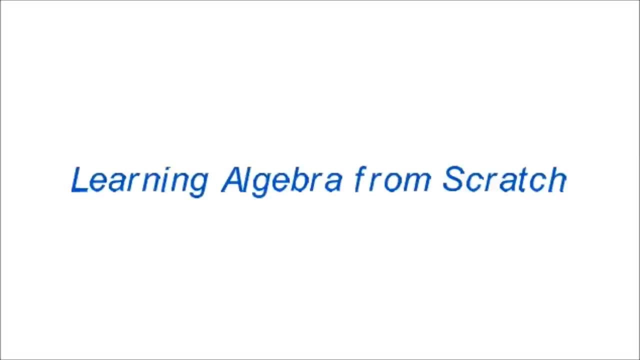 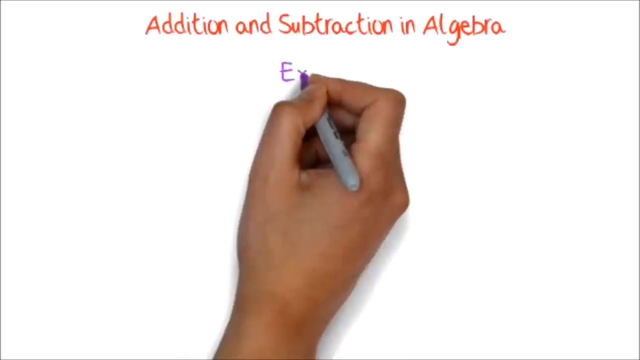 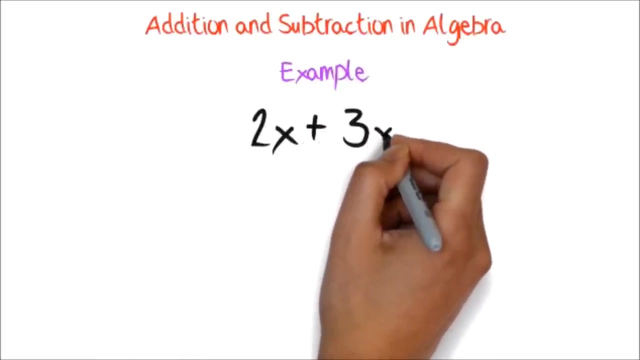 Hi, Welcome to Learning Algebra from Scratch, a course from UltimateAlgebracom. Addition and Subtractions. in Algebra We can only add things if the letters and their exponents following them are exactly the same. Example: We can add 2x and 3x because they both have x following the numbers. 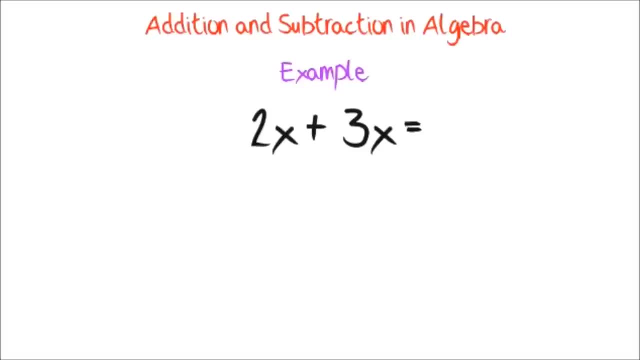 All you do is add the numbers and bring the common letter after the number. So we added the 2 and the 3 to get 5.. Then we brought the x to the right, Then we added the x after it. The final answer is therefore 5x. 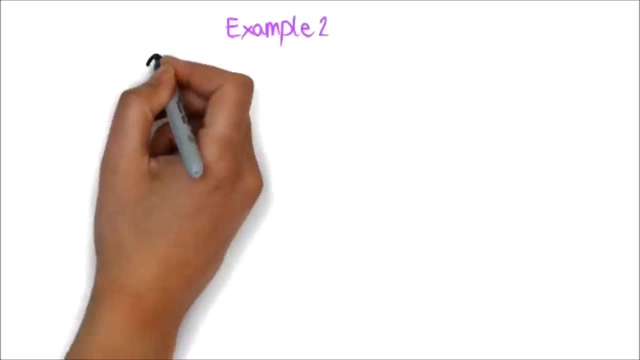 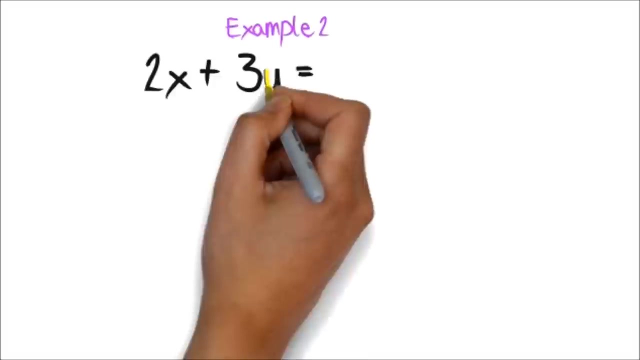 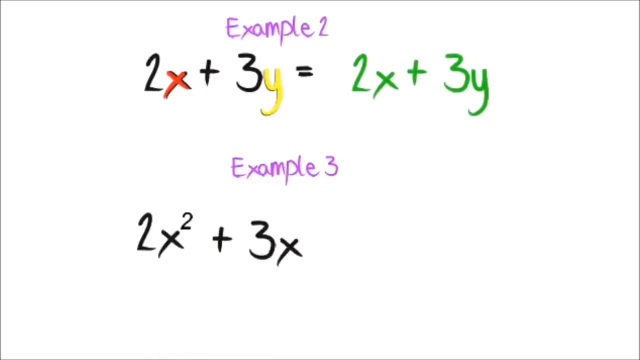 Example 2: If you have 2x plus 3y, you cannot add them because they have different letters after them. One is y and the other is x, But you can add x if there are no different numbers. Example 3: If you have 2x squared and 3x cubed, you cannot add them because of the different exponents. 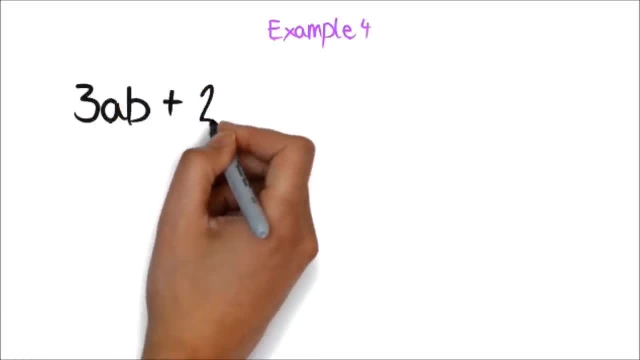 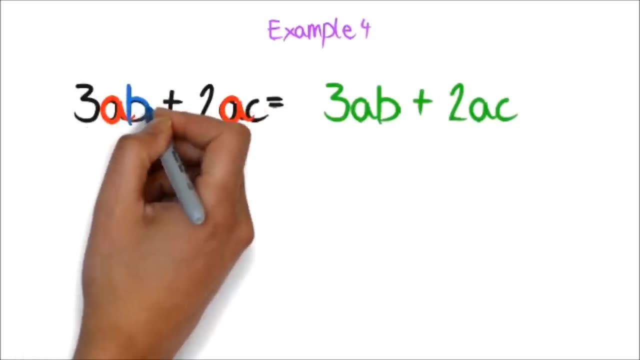 One x is squared and the other is cubed. Example: 4 plus 2 AC. although they both have a, one is a B and the other is a C. they must be exactly the same. before you can add them, let's try these: 5 a B minus 2 a B here. 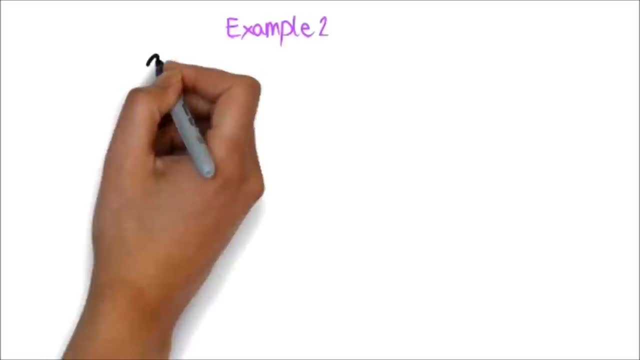 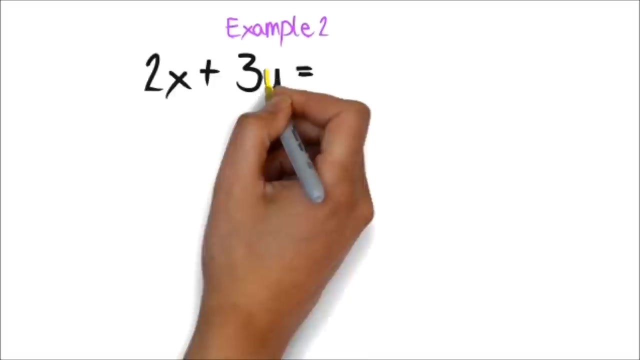 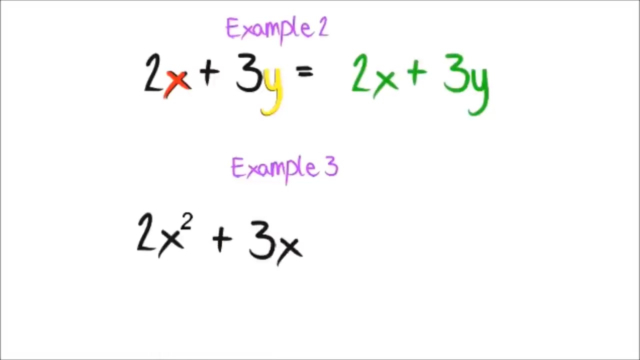 Example 2: If you have 2x plus 3y, you cannot add them because they have different letters after them: One is y and the other is x. Example 3: If you have 2x squared and 3x cubed, you cannot add them because of the different exponents. 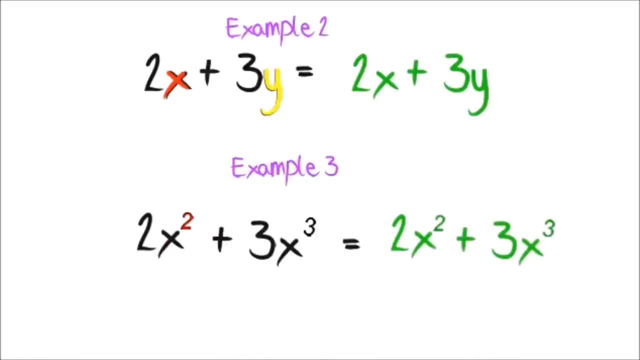 One of the x is squared and the other is cubed. Example 4: You cannot add 3ab and 4b. Example 5: You cannot add 2b and 3a. Example 6: You cannot add 3b and 3c. 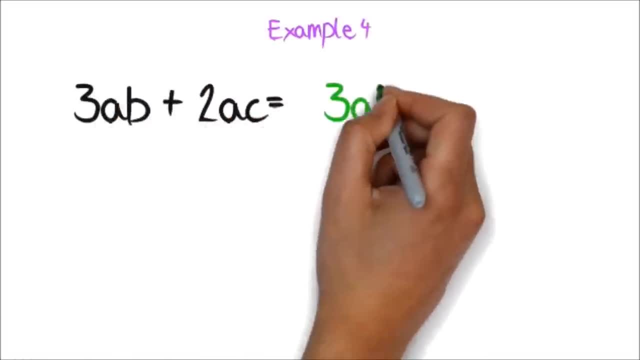 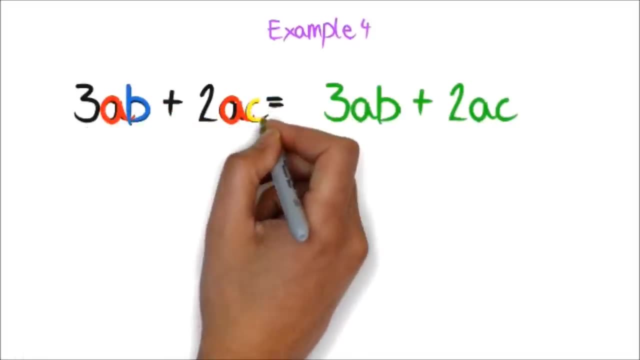 Example 7: You cannot add 3a. Example 8 plus 2 AC. although they both have a, one is a B and the other is a C. they must be exactly the same before you can add them. let's try these: 5 a B minus 2 a B here. 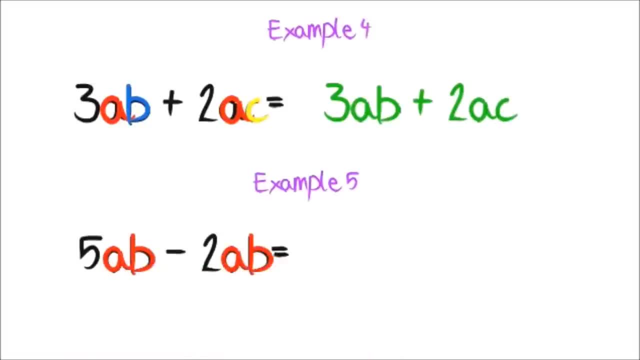 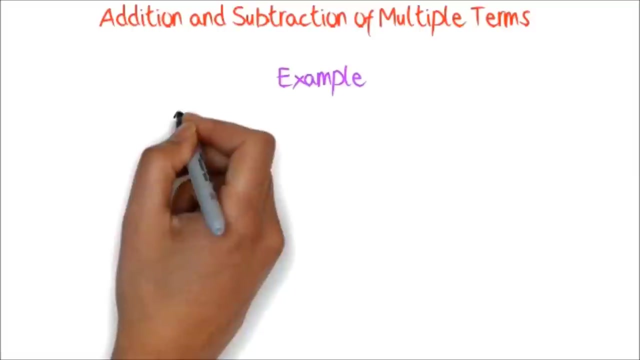 since they both have a B after the number we can subtract, this gives us 3 a B. as you can see, if your addition and subtraction is good, this should be easy addition and subtraction of multiple terms. like the way we added multiple numbers in basic math, we might have to add multiple terms in algebra. let's try this: 2 a B plus 5 BC. 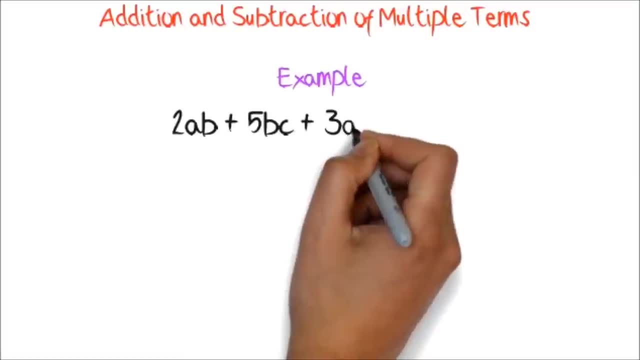 plus 3 a B minus 2 BC. here we take the first term, 2 a B, and find out if there are other terms that are equal to 2 a B, and find out if there are other terms that are equal to 2 a B and find out if there are other terms that are equal to. 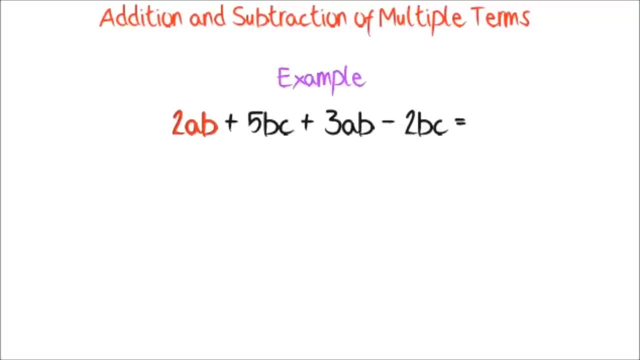 2 a B and find out if there are other terms with the same letters after it. we terms with the same letters after it. we notice we have 3 a B, so we can add 2 a B. notice we have 3 a B, so we can add 2 a B and 3 a B to get 5 a B. next we pick the. 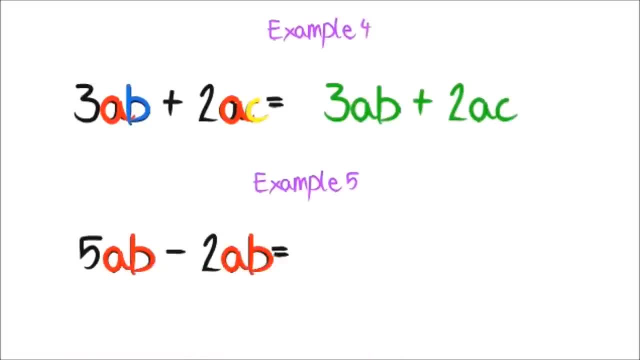 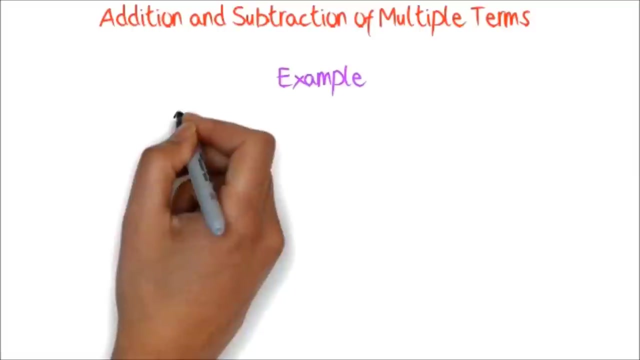 since they both have a B after the number we can subtract, this gives us 3 a B. as you can see, if your addition and subtraction is good, this should be easy addition and subtraction of multiple terms. like the way we added multiple numbers in basic math, we might have to add multiple terms in algebra. let's try this: 2 a B plus 5 BC. 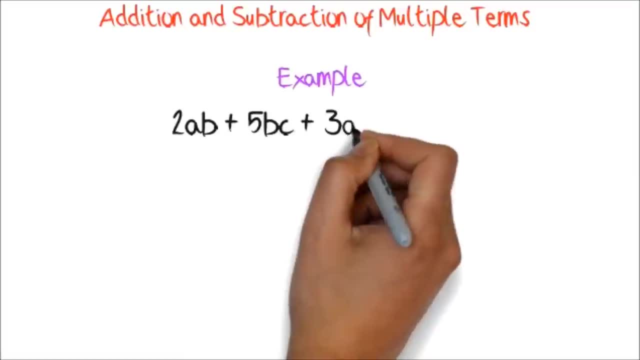 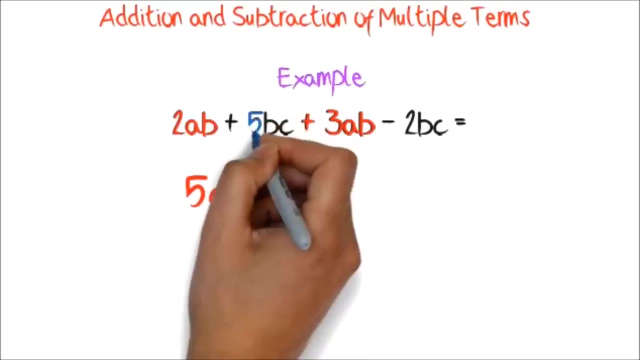 plus 3 a B, minus 2 BC. here we take the first term, 2 a B, and find out if there are other terms with the same letters after it. we notice we have 3 a B, so we can add 2 a B and 3 a B to get 5 a B. next we pick the 5 BC. we look for another term with BC. 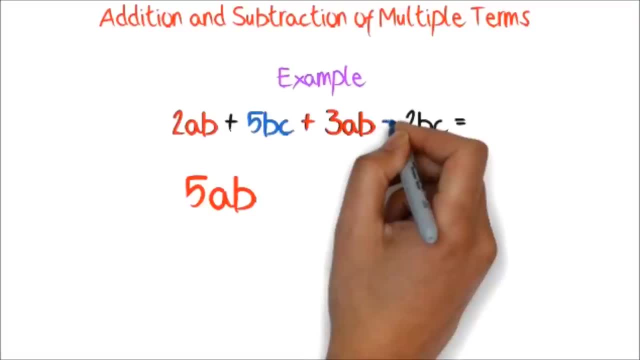 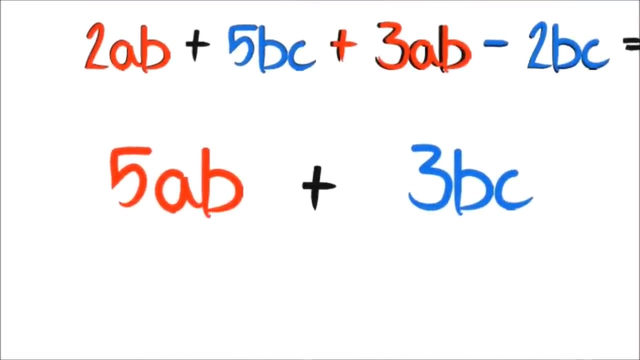 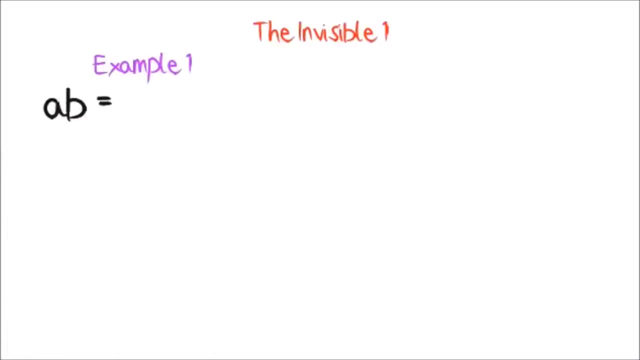 here we have negative 2 BC. we work on 5 BC minus 2 BC to get 3 BC. we cannot add 5 a, B and 3 BC since they have different letters after them. so that is our final answer, the forgot sorry. so what we are losing key is 2 a B and 3 BC is the same. we subtract 1 a B out of 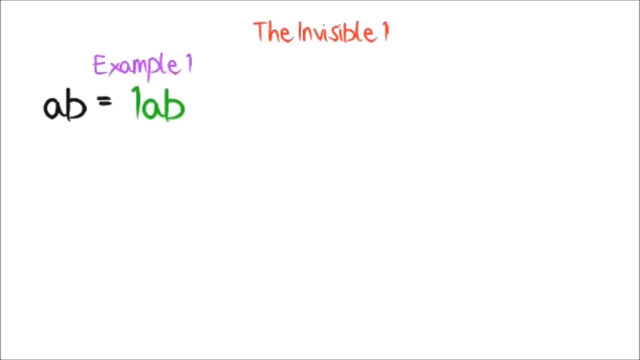 $14 and 2 a B is the same. we subtract 5 BC from 2 BC and 3 BC is the same. we have 3 a B plus 5 BC minus. what isyd the last answer? we swing different numbers before fruit and vegetables. 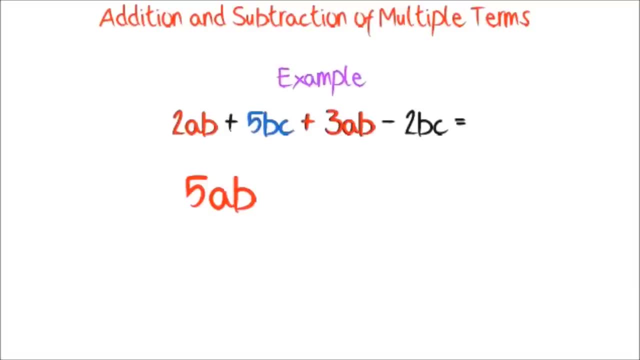 and 3 a B to get 5 a B. next we pick the 5 BC. we look for another term with BC. here we have 5 BC. we look for another term with BC- here we have 5 BC. we look for another term with negative 2 BC. we work on 5 BC minus 2 BC to get 3 BC. we cannot add 5 a B and 3 BC. 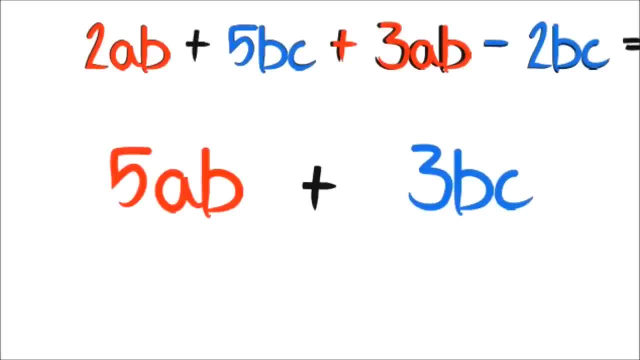 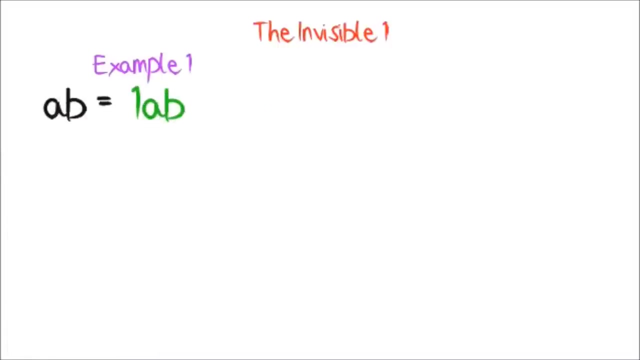 negative 2 BC. we work on 5 BC minus 2 BC to get 3 BC. we cannot add 5 a, B and 3 BC since they have different letters after them. so that is our final answer: negative 2 BC. we work on 5 BC and 3 BC to get 3 BC and 3 BC. the first. 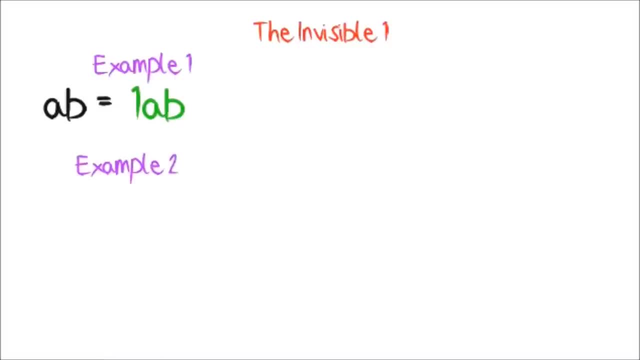 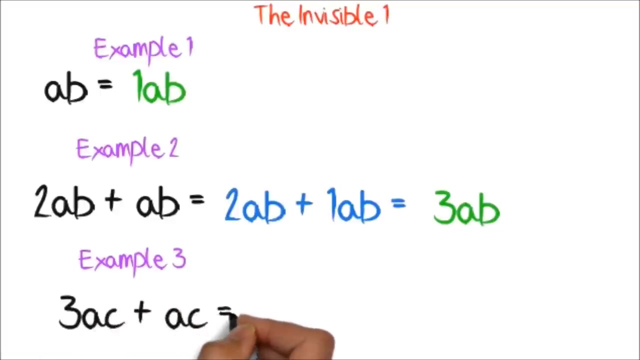 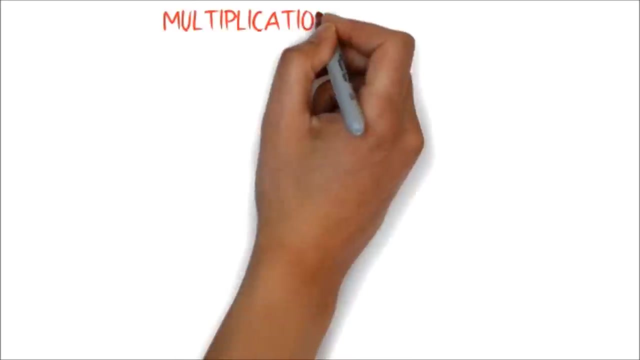 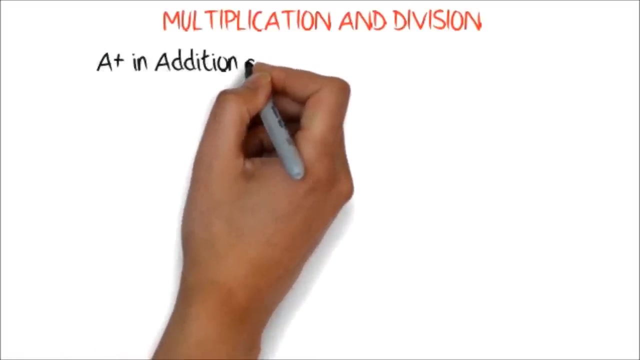 backwards as as as as equals 2 AB plus 1 AB, which equals 3 AB. again, 3 AC plus AC will be equal to 4 AC, because AC is the same as 1 AC. multiplication and division. we are now familiar with addition and subtraction. 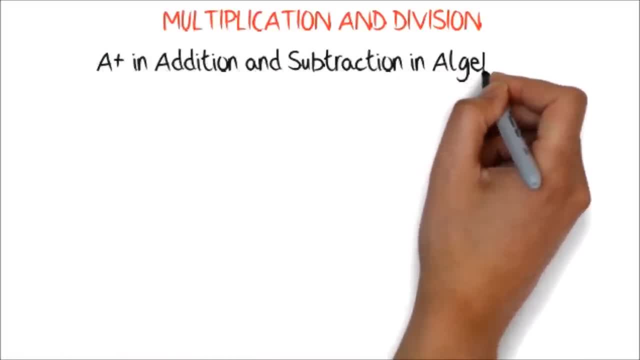 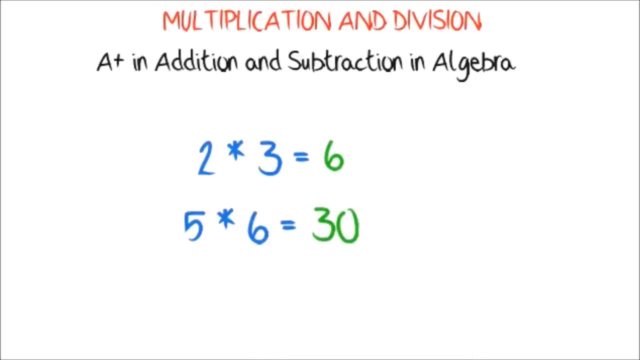 in algebra, please. I hope you have mastered it because it is a step-by-step course and we have carefully chosen the trend to make you good in algebra. I'm sure you can do these. what is 2 times 3? what is 5 times 6? if you had 6 and 30, we are good to go. if you are not good at 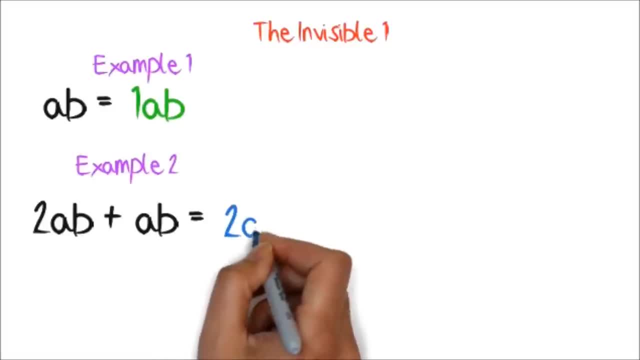 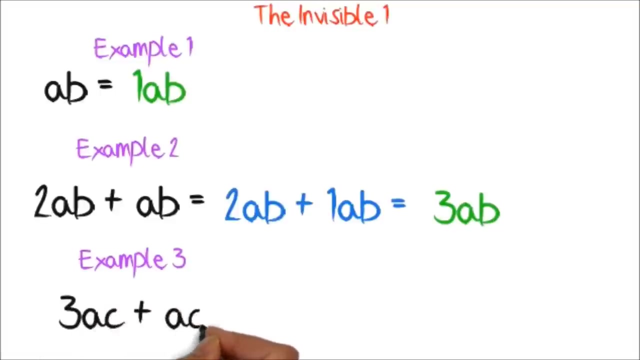 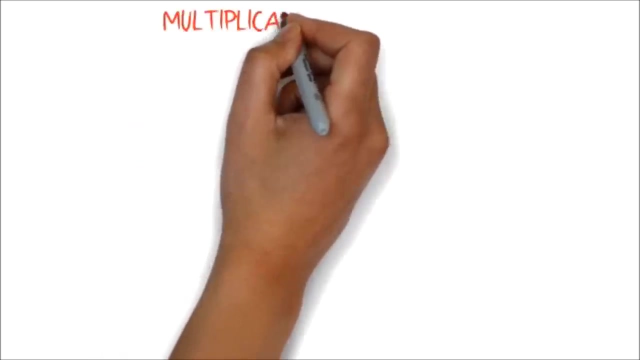 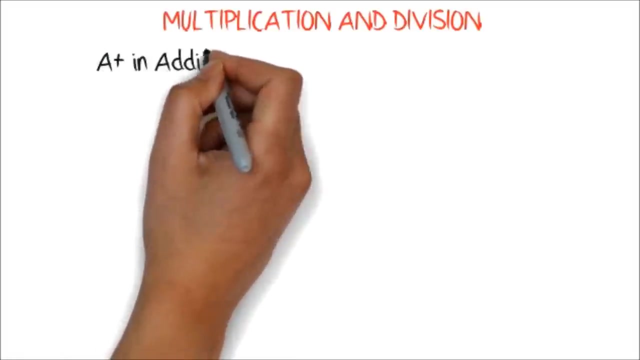 example, equals 2ab plus 1ab, which equals 3ab. Again, 3ac plus ac will be equal to 4ac, because ac is the same as 1ac. Multiplication and division. We are now familiar with addition and subtraction. 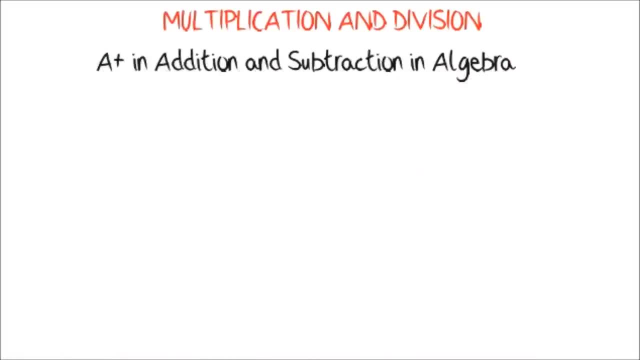 in algebra, Please. I hope you have mastered it, because it is a step-by-step course and we have carefully chosen the trend to make you good in algebra. I'm sure you can do these. What is 2 times 3?? What is 5 times 6?? If you had 6 and 30,? 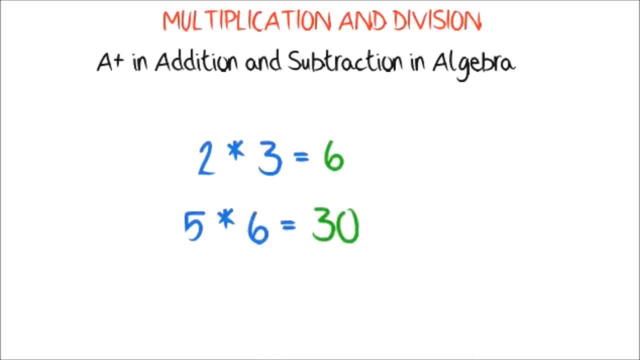 we are good to go. If you are not good at multiplication, you can either learn them later by memorizing the multiplication table or by using the multiplication table. You can use the multiplication table or by deriving it, or by watching our videos on math tricks for multiplication. 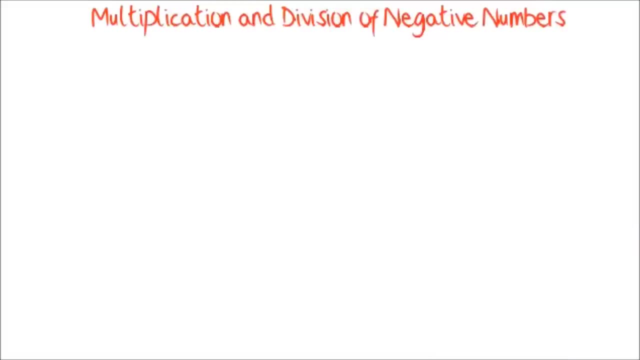 Multiplication and division of negative numbers. The real problem in most cases is when negatives are introduced. When you multiply a negative and a positive number, the answer is always negative. When you multiply a negative and a positive number, the answer is always negative. 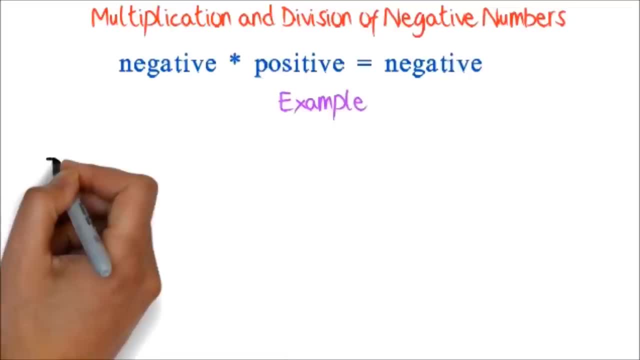 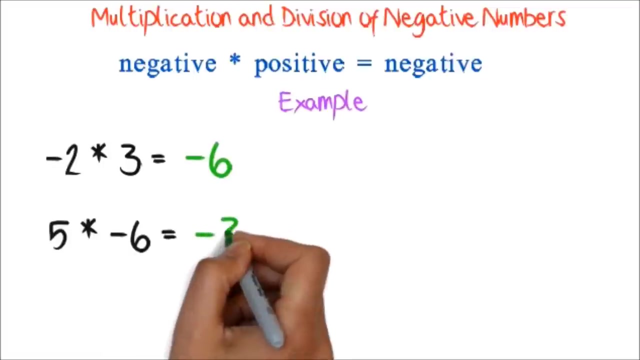 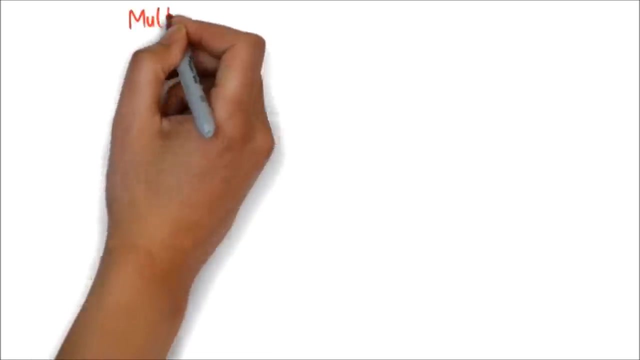 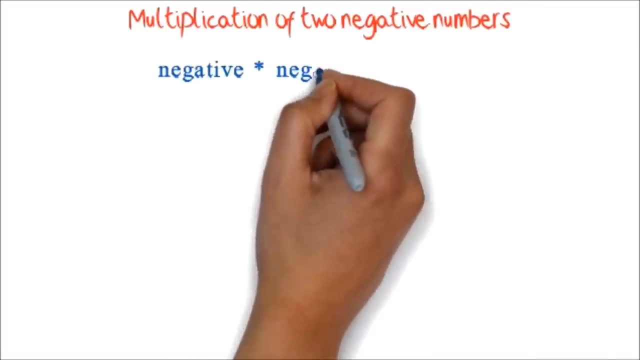 Example: negative 2 times 3 equals negative 6.. Five times negative 6 equals negative 30. Notice, in both cases one is positive and the other is negative. Now looks like the answer is negative or positive. let's look at when you multiply two negative numbers, when you multiply two negative numbers. 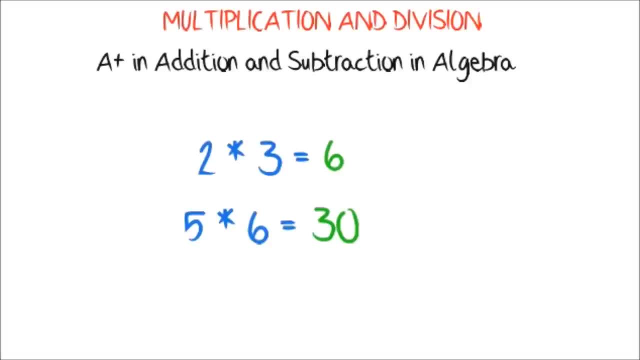 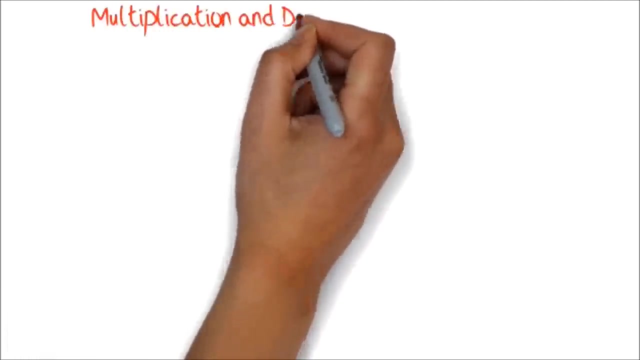 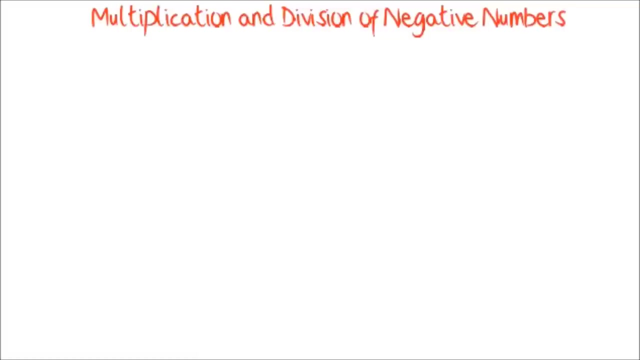 multiplication. you can either look at the multiplication table or look at the. learn them later by memorizing the multiplication table or deriving it, or watching our videos on math tricks for multiplication, multiplication and division of negative numbers. the real problem in most cases is when negatives are introduced. when you multiply a negative and a positive number. 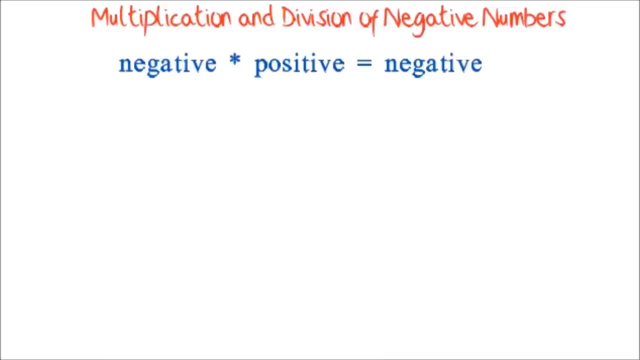 the answer is always negative. example: negative: 2 times 3 equals negative 6. 5 times negative: 6 equals negative 30. notice: in both cases one is positive and the other is negative. now let's look at when you multiply two negative numbers. when you multiply two negative numbers, the answer is always positive. so we say: 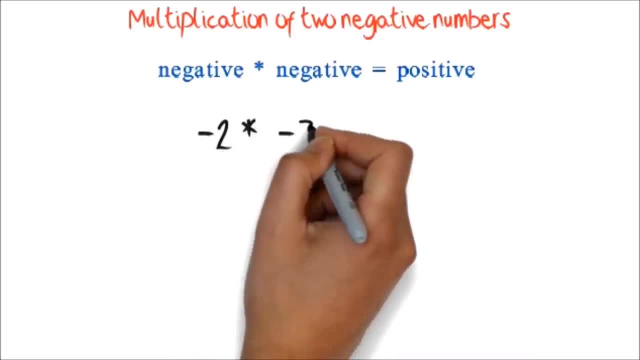 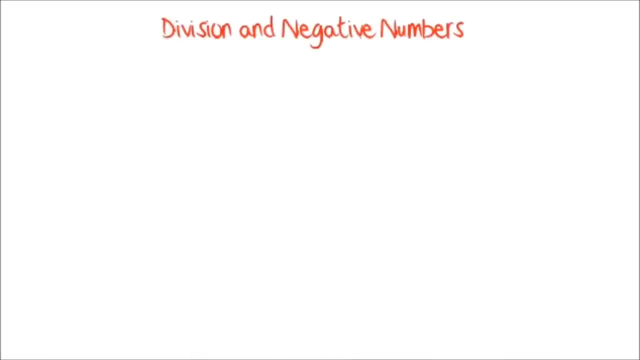 negative 2 times negative 3 equals 6 and negative negative 3 equals 6 and 5 times negative 6 equals 30.. The exact same idea applies to division. We say: negative 6 divided by negative 2 equals 3.. Notice, we worked with two negative numbers and our final answer is positive. 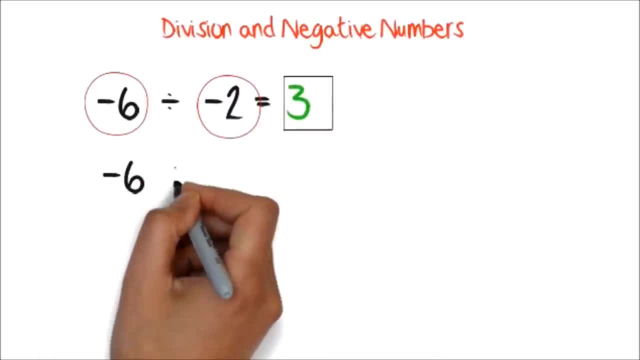 When we divide negative 6 by 2, we get our final answer to be negative 3.. Here one of the numbers is negative and the other is positive. 6 divided by negative 2 will give us negative 3.. Here again, 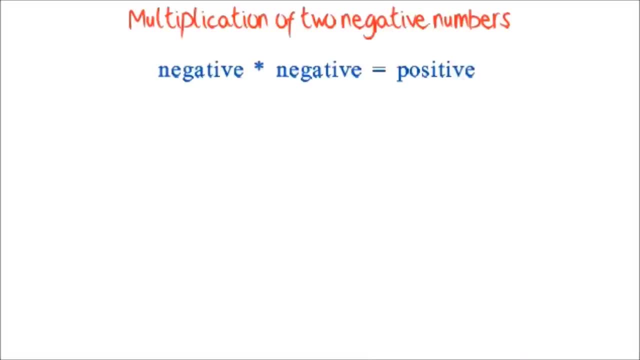 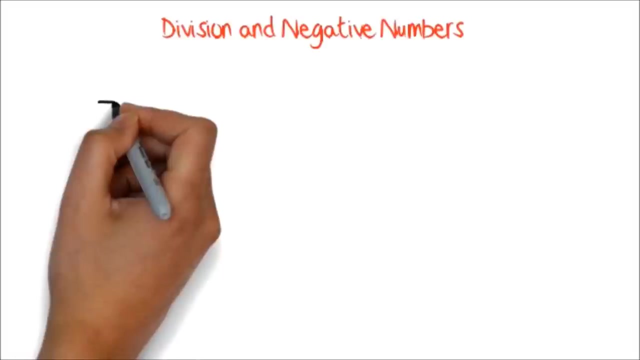 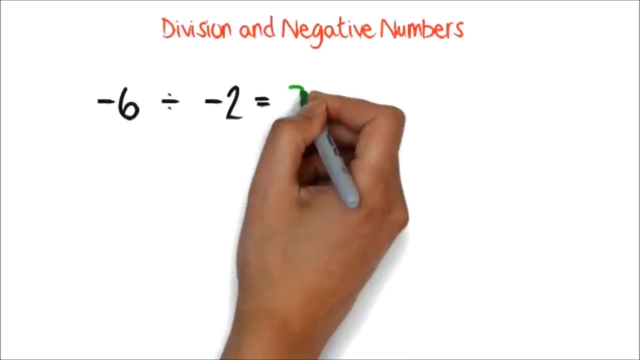 the answer is always positive. so we say: negative 2 times negative 3 equals 6 and negative 5 times negative 6 equals 30. the exact same idea applies to division. we say: negative 6 divided by negative 2 equals 3. notice, we worked with two negative numbers and our final answer is positive. 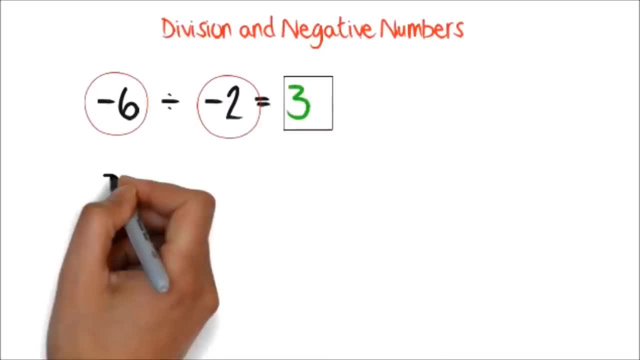 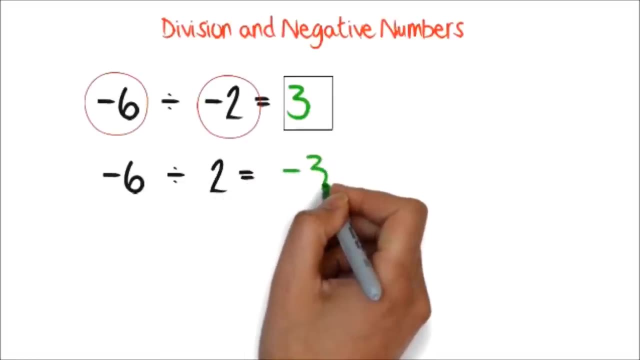 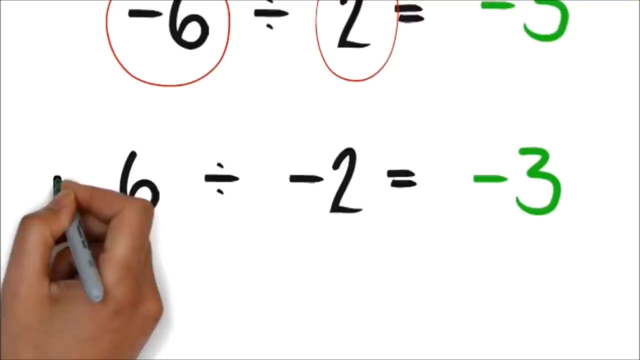 when we divide negative 6 by 2, we get our final answer to be negative 3. here one of the numbers is negative and the other is positive. 6 divided by negative 2 will give us negative 3. here again, one of the numbers is positive and the other is negative. 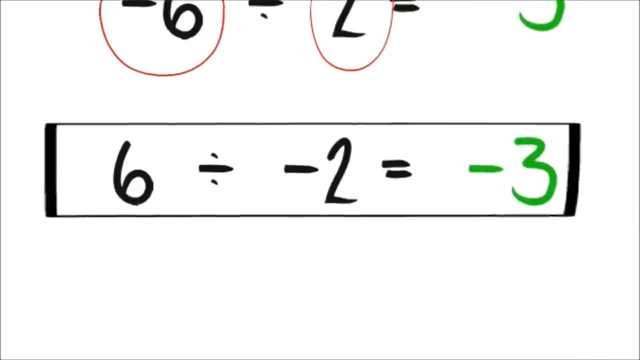 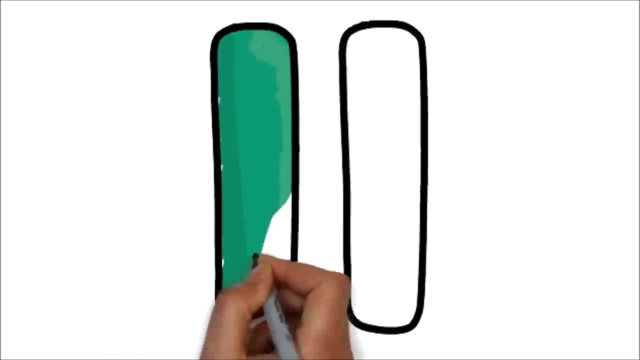 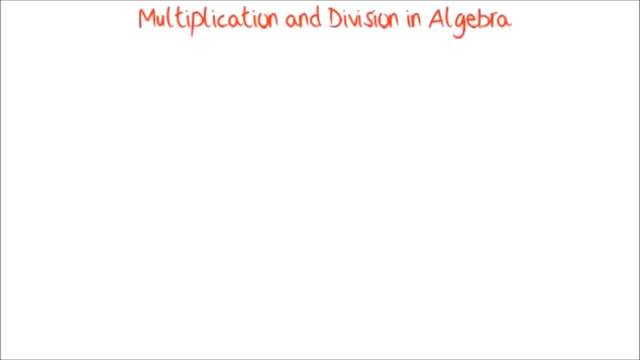 so our final answer is negative. please pause this video and make sure you are familiar with the multiplication and division of negative numbers before we move on multiplication and division in algebra. when we learnt addition and subtraction in algebra, we said that letters must be exactly the same before you can add or subtract them. 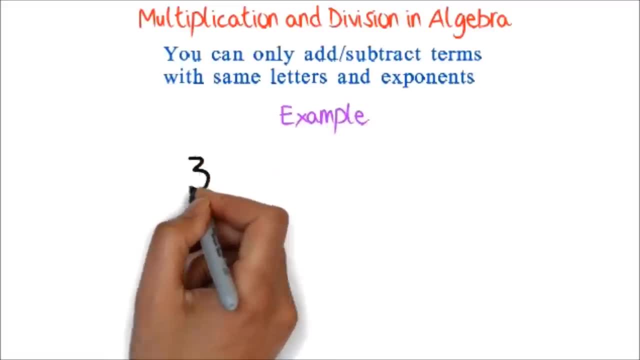 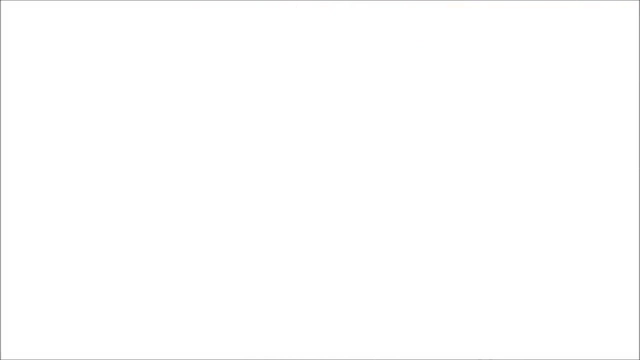 example, we can add 3a and 2a because both have the same letters after the number. we also said we can't GE. the first thing you'll do is multiply the numbers, the numbers, just like we did in basic math. multiply the 6 and the 2 to get 12. now for the. 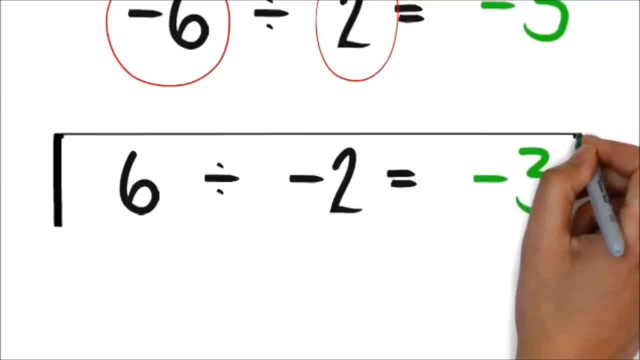 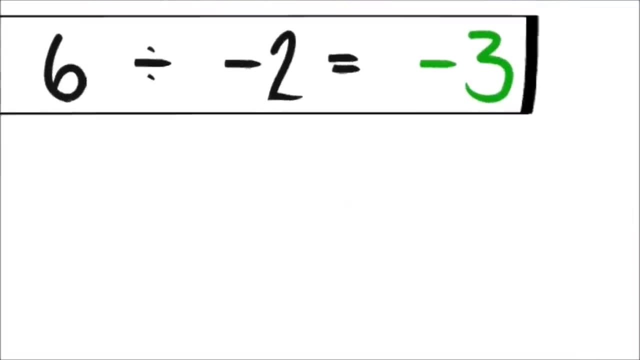 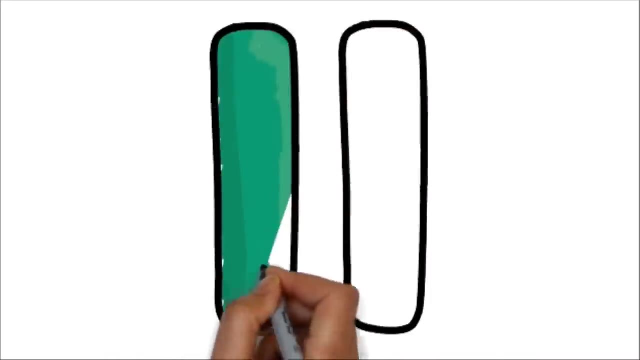 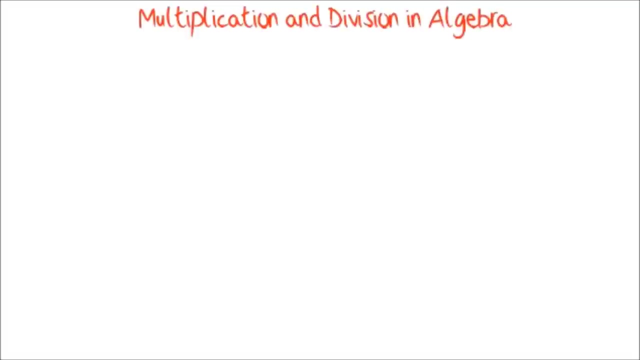 one of the numbers is positive and the other is negative, so our final answer is negative. Please pause this video and make sure you are familiar with the multiplication and division of negative numbers before we move on. Multiplication and division in algebra: When we learned addition. 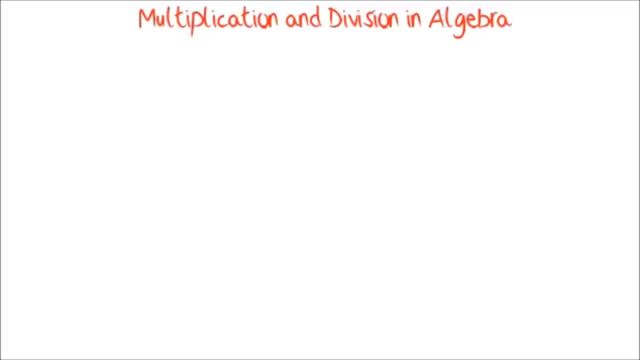 and subtraction. in algebra we said that letters must be exactly the same before you can add or subtract them. we can add 3a and 2a because both have the same letters after the number. We also said we cannot add 3a and 2b because the letters 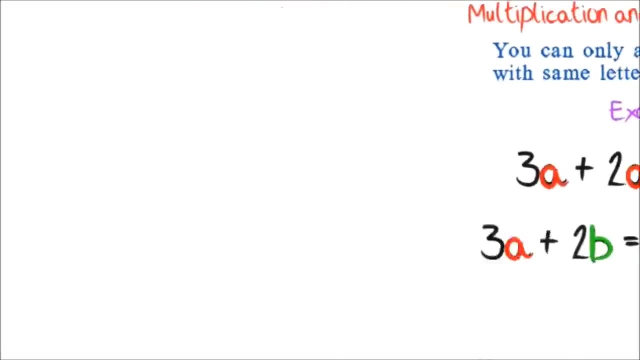 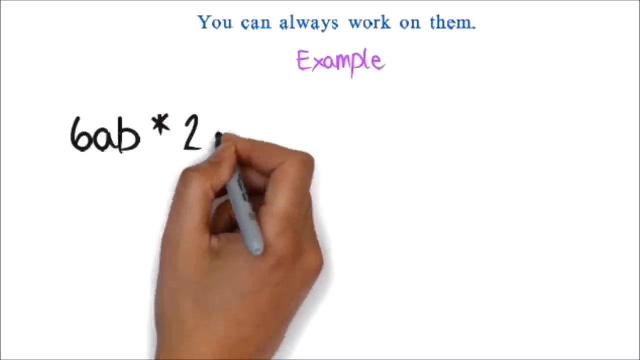 are different For multiplication and division. it doesn't matter. the letters can always work on them. example: 6ab times 2ac. the first thing you'll do is multiply the numbers, just like we did in basic math: multiply the 6 and the 2 to: 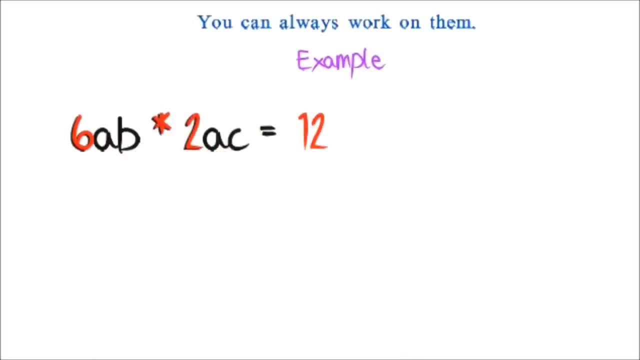 get 12. now for the letters. we just look at the number of occurrences here, we can see that there are two A's, so we have a exponent 2. there is just one B, so we have B here and we also have one C. easy, right, let's try these negative 3ab times. 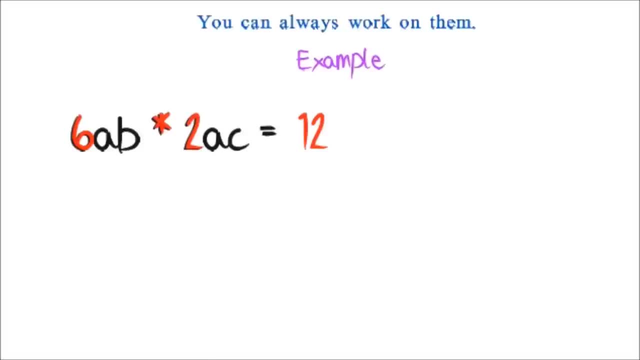 letters. we just look at the number of occurrences here, we can see that there are two A's, so we have a exponent 2. there is just one B, so we have B here and we also have one C. easy right, let's try these negative 3 a, B. 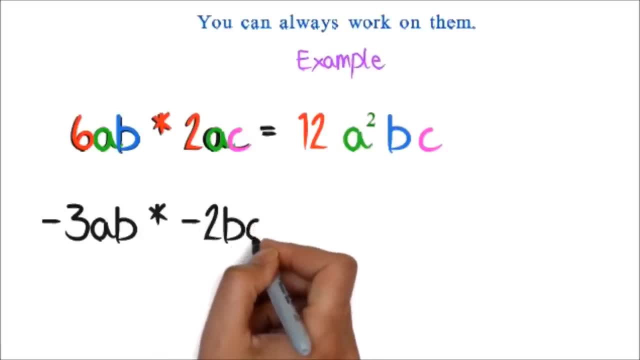 times negative: 3 a B times negative. 3 a B times negative two b, c. here we multiply the negative three and negative two. these are both negatives, so we have positive six. next we look at the occurrence of the letters. the a occurs just once, the b occurs twice and the c occurs once. so our final answer is 6 a b squared c. 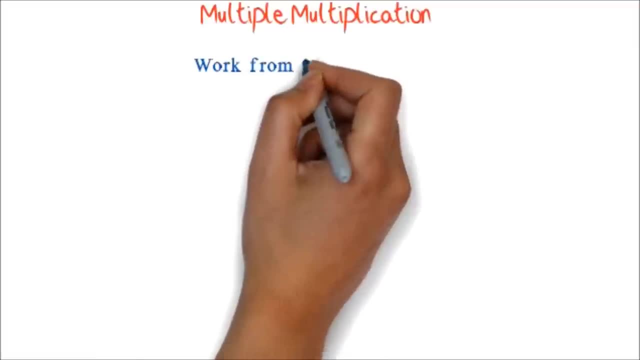 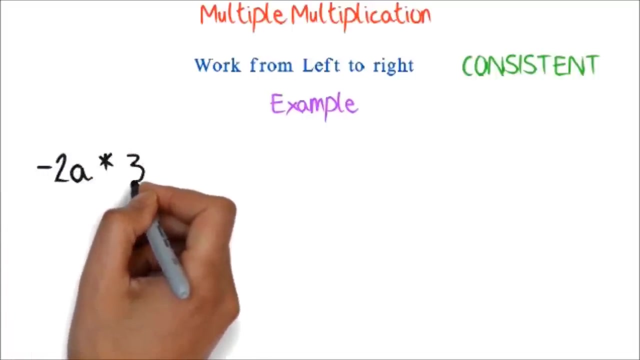 when dealing with a lot of multiplications, please work on them from left to right. this is not a mathematical requirement. this will just make it consistent with operations like division and subtraction that require that order. example: negative 2 a times 3 a. b times 2 b. 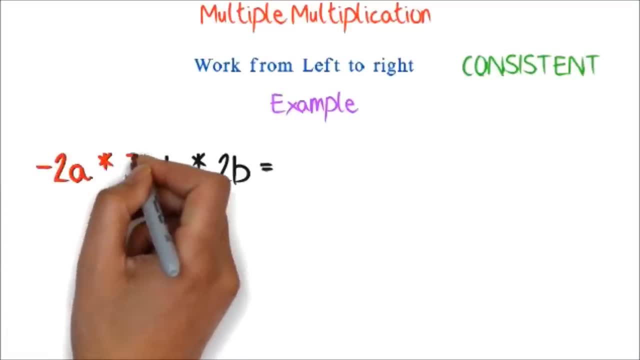 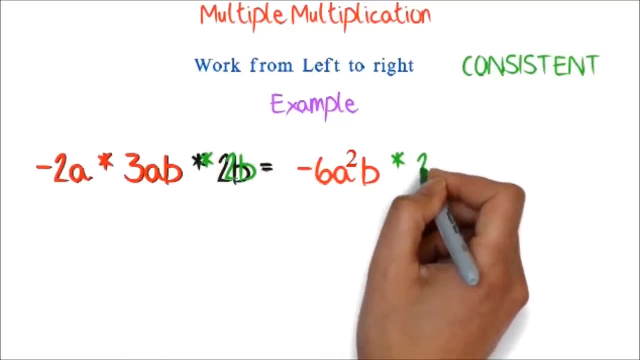 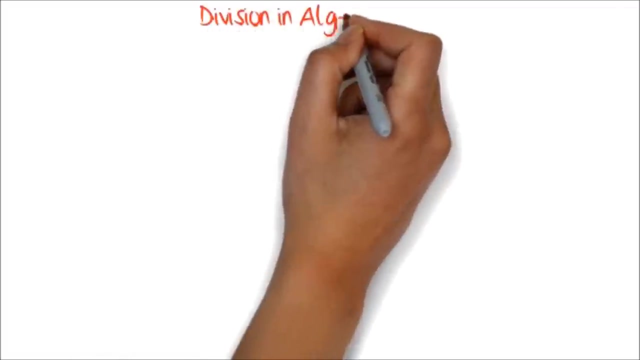 here we will do the negative 2 a times 3 a, b first to get negative 6 a squared b. then we'll multiply this by the 2b to get negative 12 a squared b. squared division in algebra in division. we are still looking at occurrence. 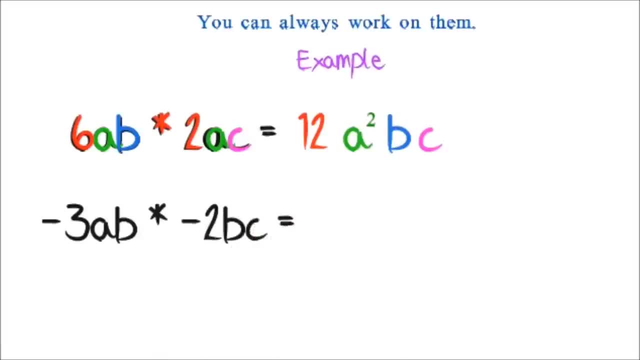 negative 2bc. here we multiply the negative 3 and negative 2. these are both negatives. so we have positive 6 negative. we look at the occurrence of the letters. the a occurs just once, the B occurs twice and the C occurs once. so our final answer is 6 a B squared C. when dealing 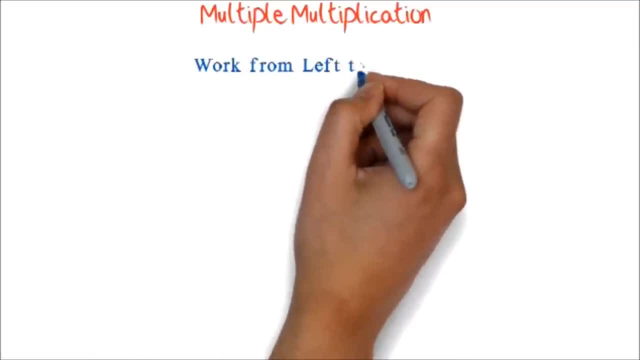 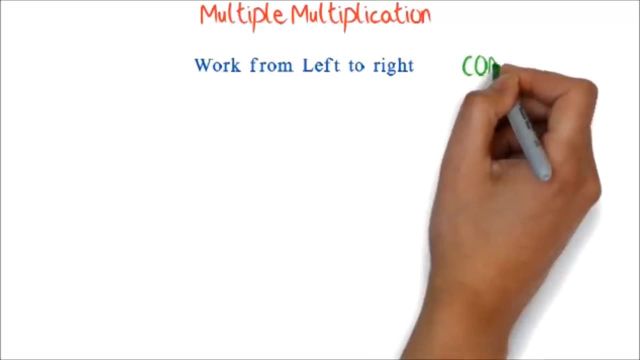 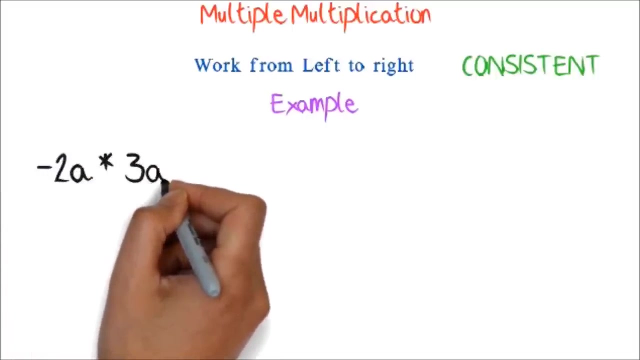 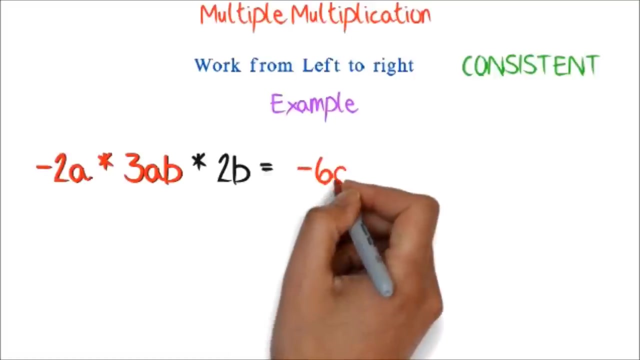 with a lot of multiplications. please work on them from left to right. this is not a mathematical requirement. this will just make it consistent with operations like division and subtraction that require that order. example: negative 2a times 3ab times 2b. here we will do the negative 2a times 3ab first to get negative 6a squared B, then we'll. 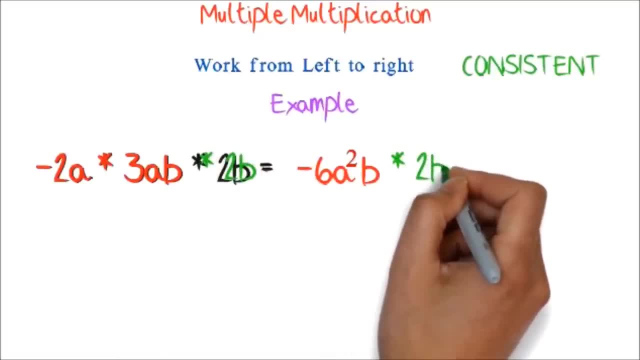 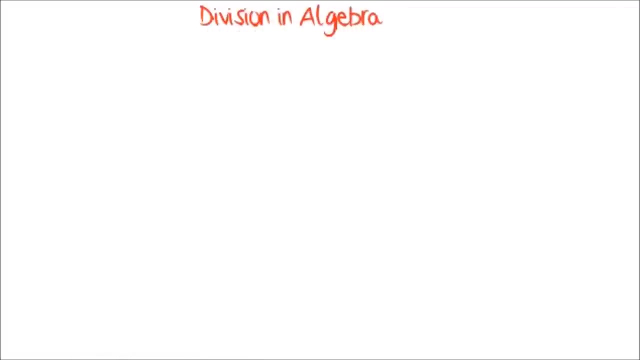 multiply this by the 2b to get negative 12 a squared- B squared division. in algebra, in division we are still looking at occurrence, but in a slightly different way. let's look at 6 a squared B divided by a negative two a, B squared. I will encourage you to write it in the: 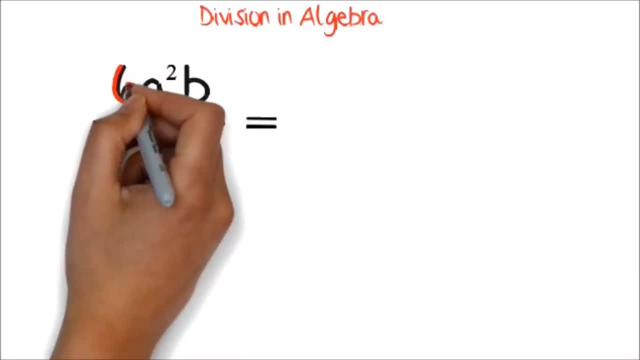 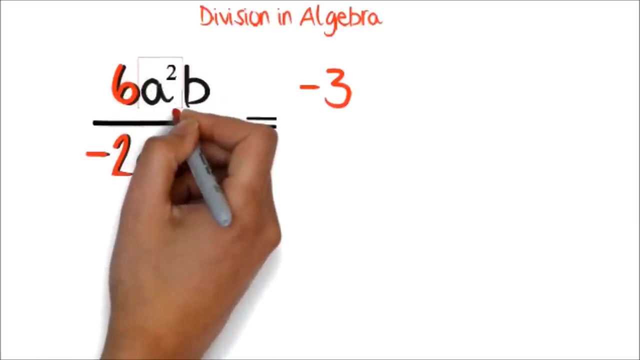 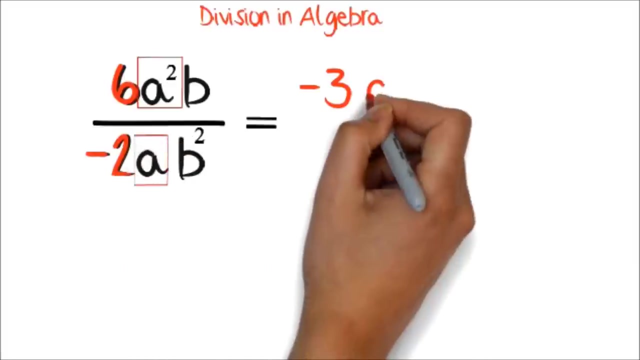 fraction form. it is easier. we divide the numbers as you ground. we divide the 6 by negative 2 to get negative 3. now we say there are two A's at the top and one at the bottom, so there will be one left at the top, there is one B at the top and there are two. 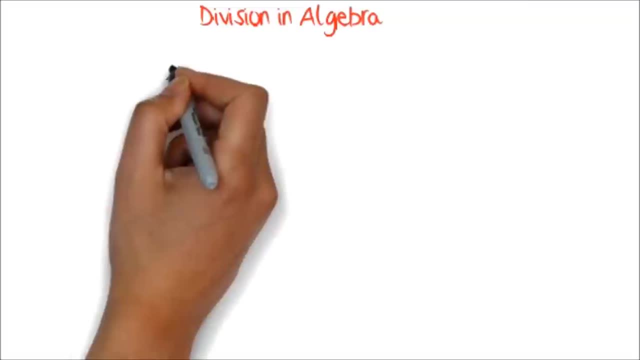 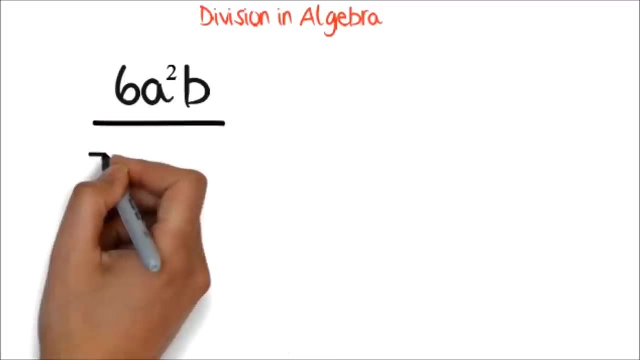 in a slightly different way. let's look at 6 a squared, b divided by negative. 2 a b squared. i will encourage you to write it in the fraction form. it is easier. we divide the numbers as usual. we divide the 6 by negative 2. 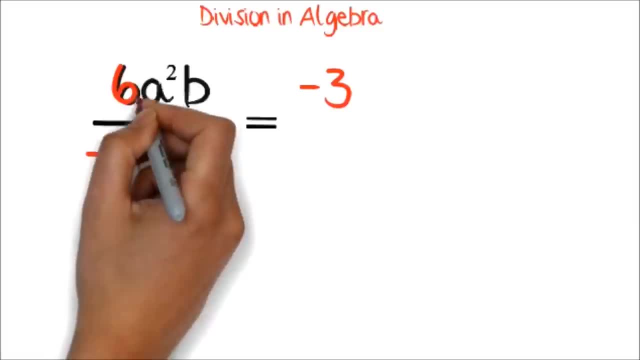 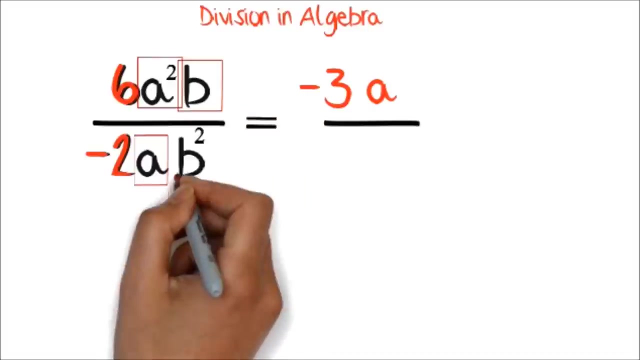 to get negative 3. now we say there are two a's at the top and one at the bottom, so there will be one left at the top. there is one b at the top and there are two at the bottom, so there will be one left at the bottom. what we are actually doing is this: a squared. 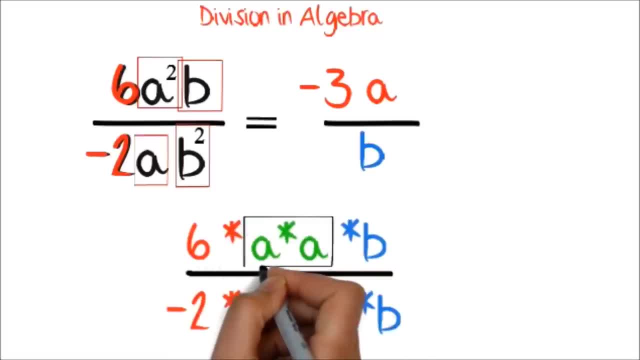 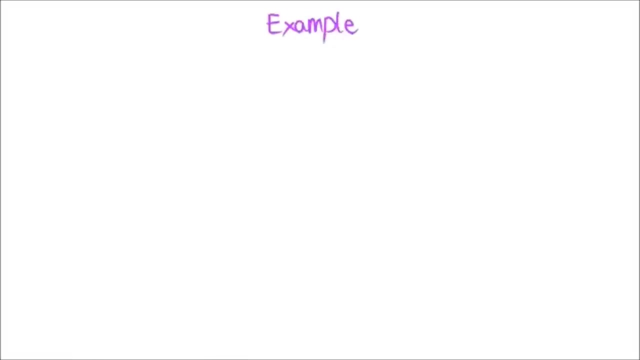 is the same as a times a. so we are just splitting the exponents and cancelling the common letters. notice that we did the same for the b. after the cancellation, we notice that we have one a at the top and one b at the bottom. if you look at your calculator, we already have two a's and b squared. 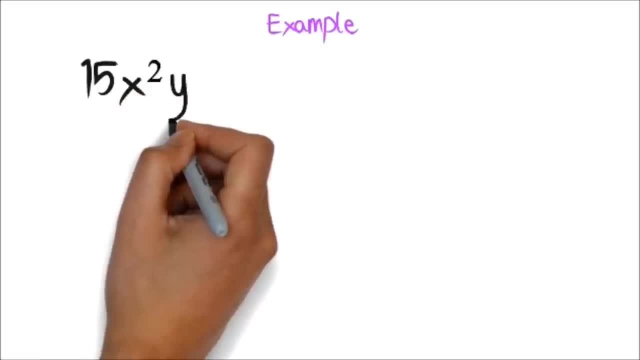 so every time you write a function you have to get the same number of elements. you can see here, for example, that we speak in a participle, so the number, THE jamais, is 12 x 2 x in our text, and now we're going to write the fifty z, final, gez, who has 2 a's and 2 x squared. 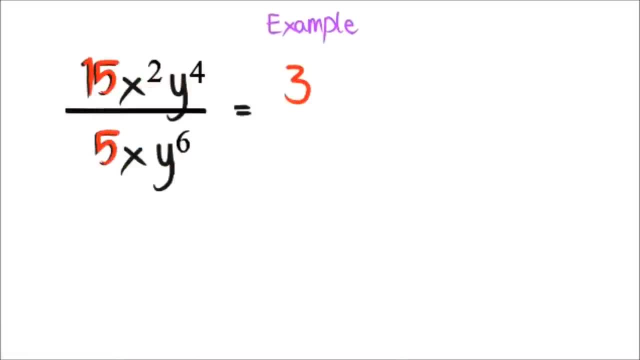 so you will plug in the kingommt and the number z to get negative 7 x squared, and when we write the negative 5x we will: okay, awesome, the top and one at the bottom. so our answer will have one X at the top also. 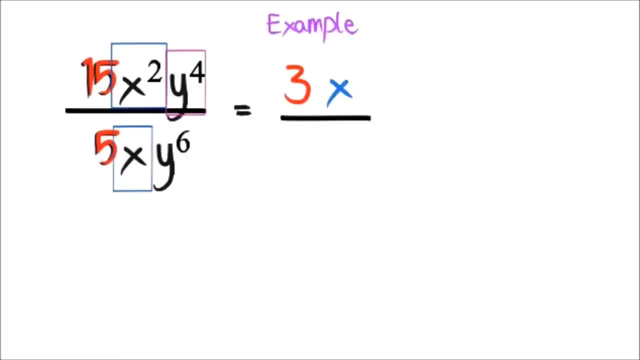 we see there are four wise at the top and there are six wise at the bottom. so there will be two wise left at the bottom. so this is our final answer.